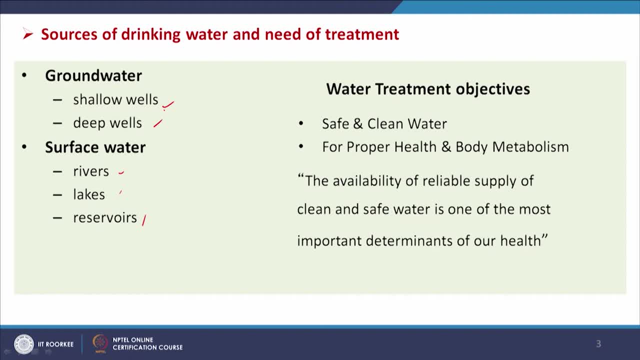 increase the well deep. if we go deeper, the wells normally becomes more safer and require less treatment, And shallow wells normally water. shallow shallow wells are used for shallow wells. water normally contains more contamination like arsenic, fluoride, etcetera, and requires more treatment. 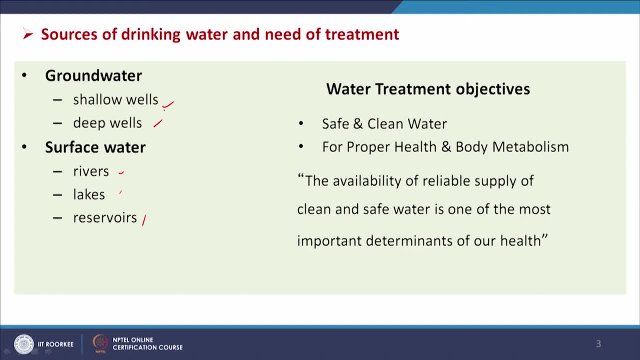 And the main objective of the water treatment for the drinking water generation is to make the water safe and clean water, to provide clean water for a proper health and body metabolism. So this is the objective: The availability of reliable supply of clean and safe water. 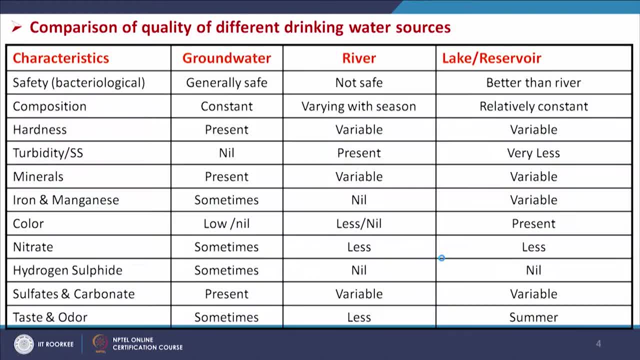 is one of the most determinants of our health. Now, if we see, there are basically some sources: one is your ground water, then river and lake or reserve here. So in these cases if we consider the characteristics, then you see that bacteriological count that is in ground 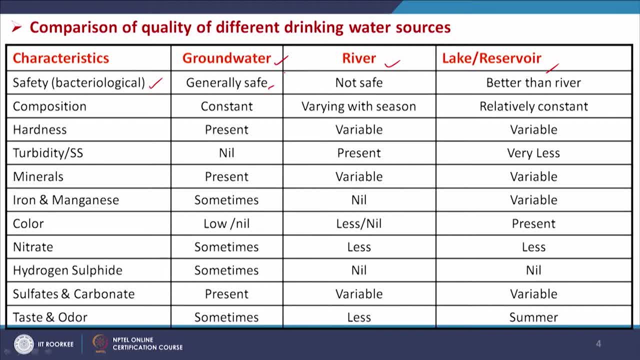 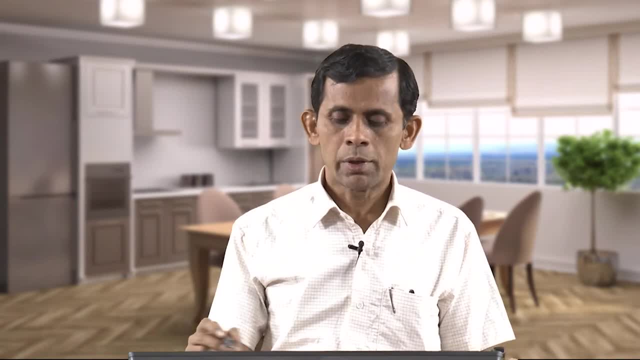 water generally it is safe and river water not safe, the more chance of contamination. So that we are just discussing that the safer source are preferably used for drinking water generation. So ground water is used in higher extent, but when the river water is not, that 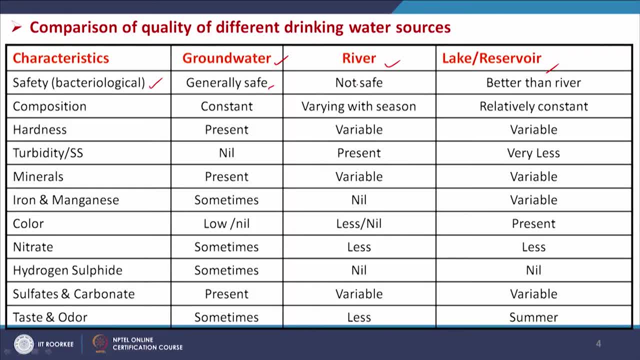 contaminated? certainly it is used and lake and reservoir water are less contaminated than river water and mostly used for drinking water. and if we see the consumptions, hardness, turbidity, minerals And iron and manganese, then color, nitrate concentration, hydrogen, sulphide and sulphates and carbonate and taste and odour, we will see that these are not equal for all three. 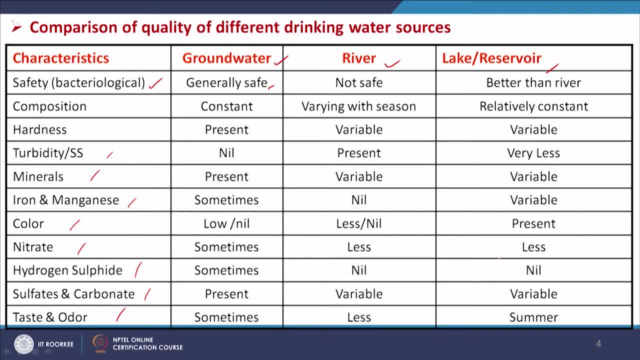 cases that means the quality of the water source is different And in case of this ground water, we will see that the hardness and different types of ions mostly available in most of the cases, And the TSS, etcetera and odour test is also. sometimes. it is available, that is sometimes. 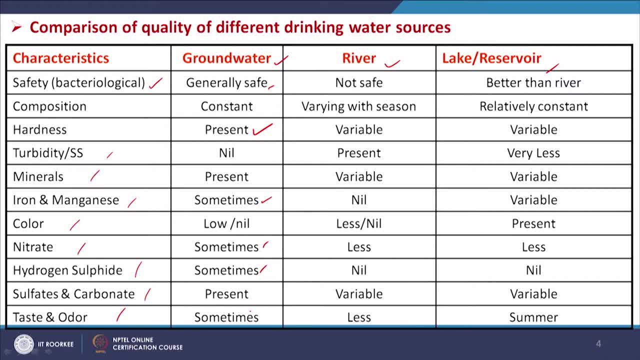 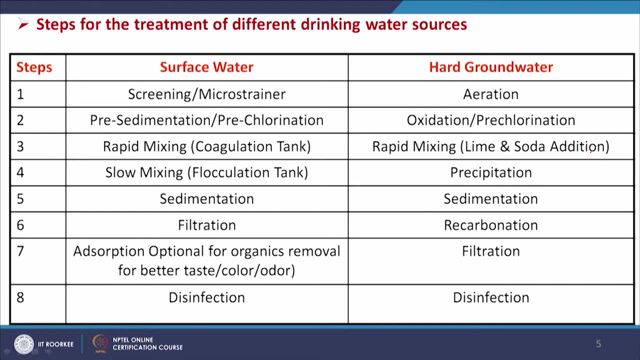 odour and taste we also get, and TSS is normally not available in the ground water, whereas this is available in river water and in reservoir water also, this is less Now if we see the steps for the treatment of different drinking water sources, then surface water and hard ground water, if we see the almost similar steps are there, but in in. 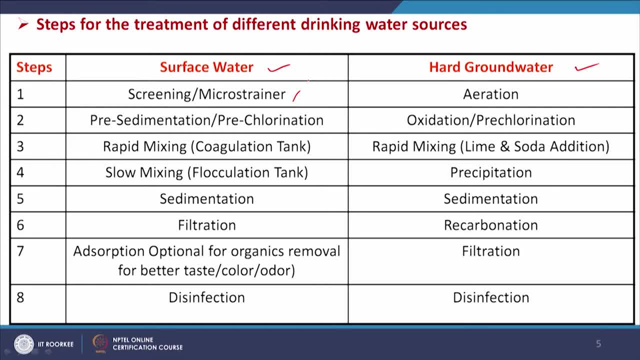 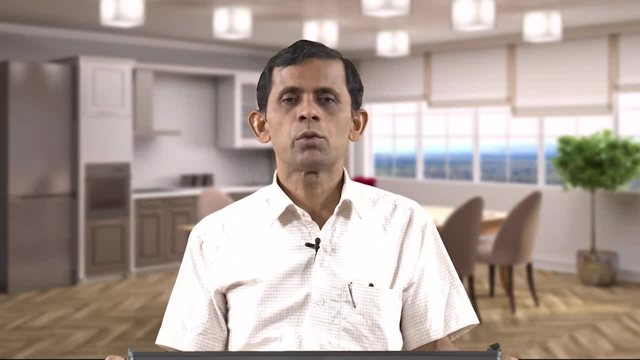 case of surface water, the skinning are micro strainer is used, but in case of hard ground water this is not required. but in some cases aeration is required because by providing oxygen some reduced form of different ions can be converted to oxidized form and can 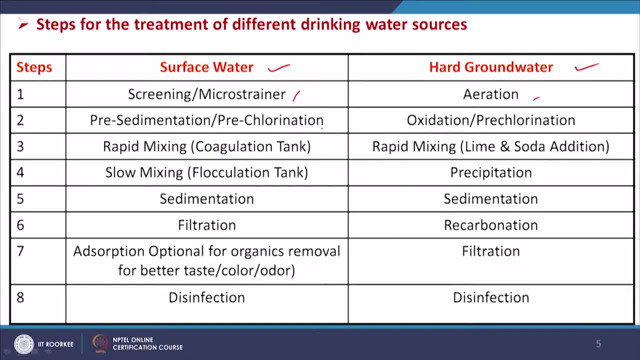 be removed easily from the ground water. Then sedimentations and pre-chlorination. and here oxidations and pre-chlorinations in case of ground water is needed just we have mentioned, to convert some ions to oxidized form that can be easily removed. 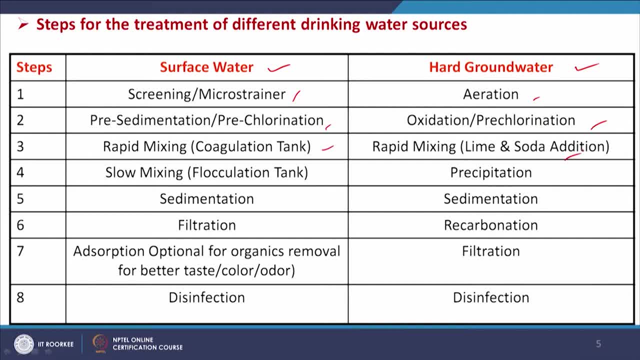 And then rapid mixings are applicable for both the cases, and then slow mixing and then sedimentation filtrations are used for surface water and where we can go for precipitation, sedimentation, recarbonation. So recarbonation is required here because in this case, as we are using lime and soda, 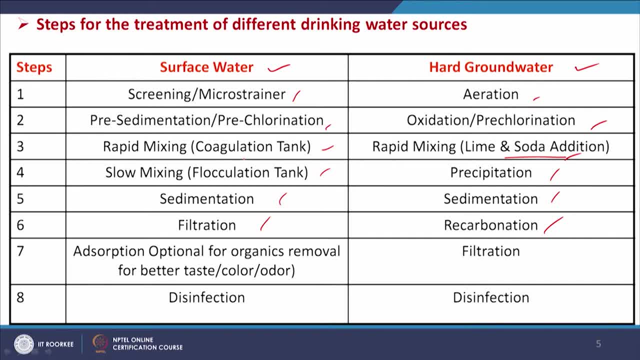 additions you see here in case of rapid mixing for surface water coagulation tank and rapid mixing lime and soda additions in case of ground water. So here the pH is increased, so carbon dioxide is again sent to reduce the alkalinity or increase the pH or to reduce the pH. 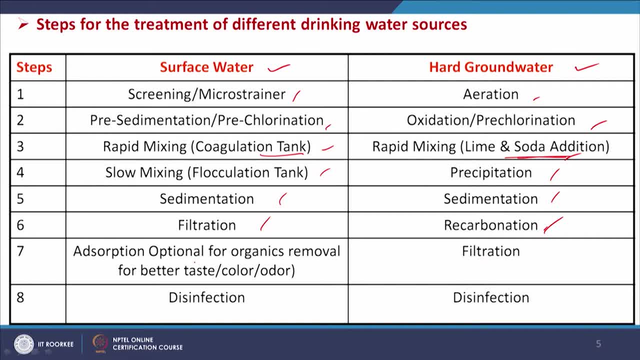 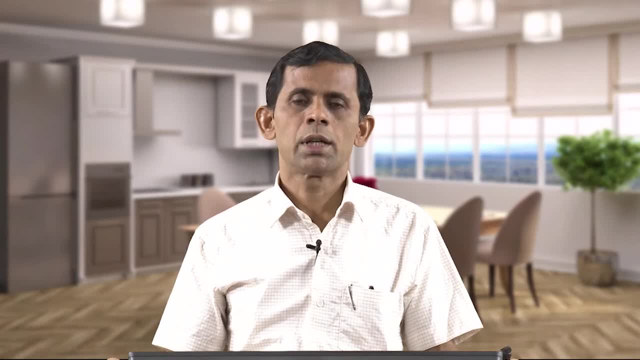 Then filtration is common for both the cases And adsorption is optional for odors, Organics removal for better taste, odor etcetera, when the we are considering the river water or reservoir water. so BOD COD may be available in this, but normally in hard ground water. 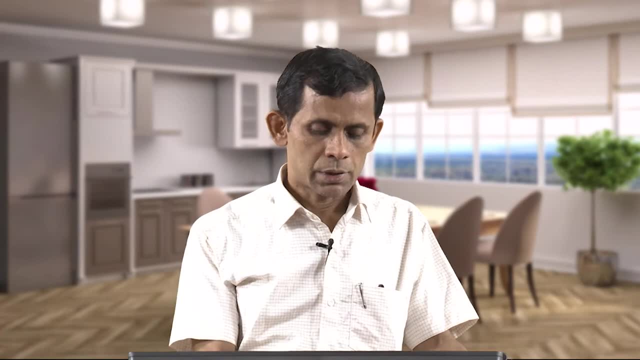 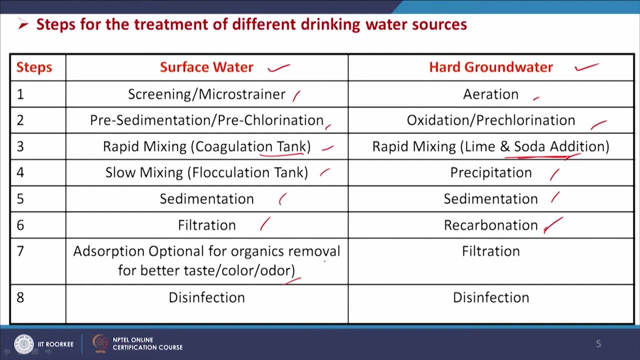 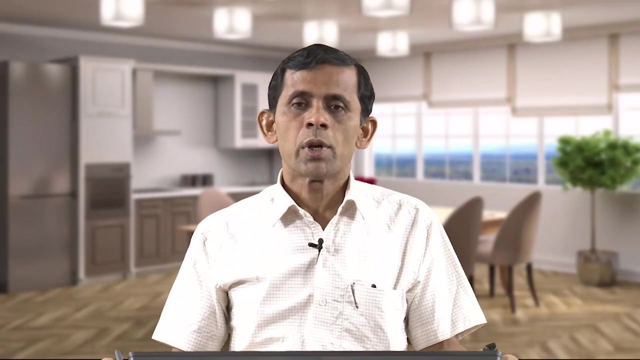 BOD COD is not available, So in that case adsorptions- optional adsorption may be made optional for organics, removal for better taste and odor and color and disinfections is common for both the sources. Disinfection is must Because the water which we will be drinking, that must be free from pathogenic microorganisms. 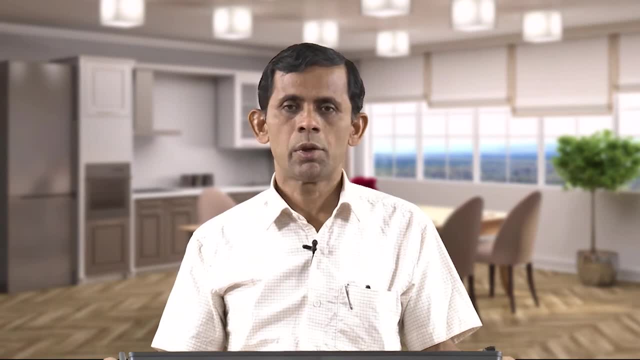 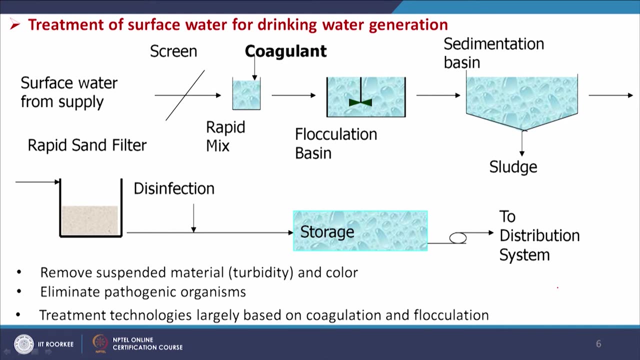 so disinfection is mandatory for all type of drinking water generation. Now we will see the surface water treatment for drinking water generation. If we see the first surface water from supply, then we have a screen, the removing of, say, floating materials like the leaves paper, piece of papers or anything like this. so then, 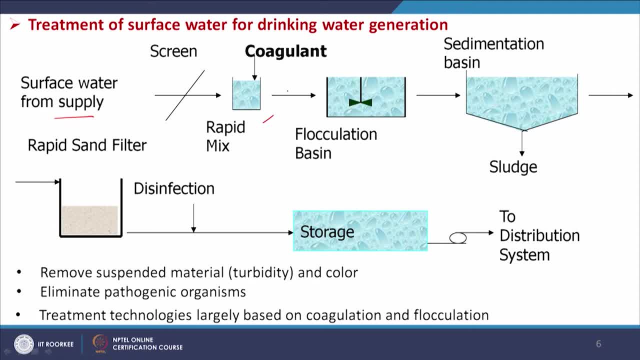 after that it will be coming to coagulant. So we will be adding some coagulant so that the BOD or COD, if it is available, or if some suspended solids, and the dissolved solids will also be settled, and then we will be adding. 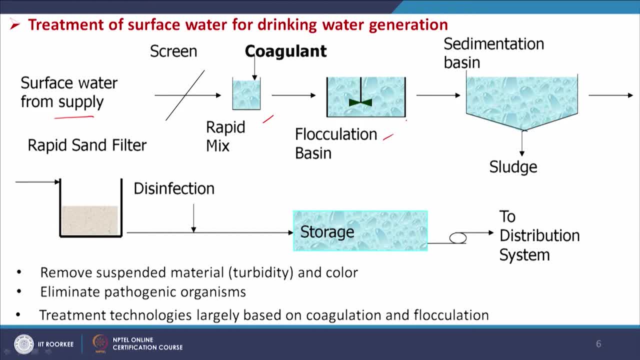 some flocculation machine. so the tiny particles, the colloidal particles, will be given an opportunity to collide each other and to make into a bigger form and settle. Then we are coming to sedimentation. So the sedimentation machines will be providing sufficient time so that the clogs which we 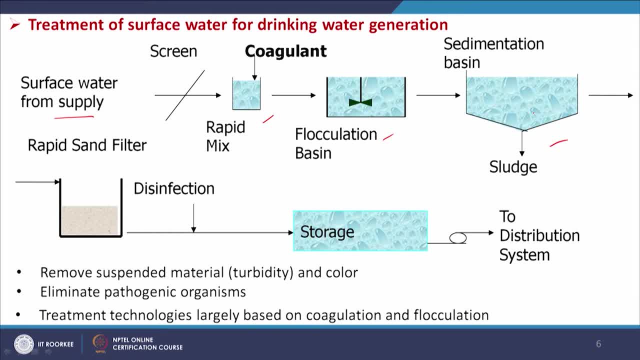 are forming, so that can be settled, and then it is coming to rapid sand filter. So sand filters will be there, then the it will be purified and then the water is ready almost for its applications. but before that disinfection is necessary to kill all the microorganisms present in it. then it will be stored and to be distributed. 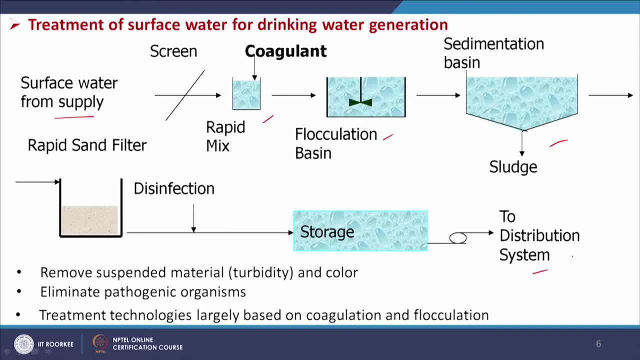 So this is the general flow sheet for the treatment, For the treatment of surface water for drinking water production, and main objective of this treatment is to remove suspended material, that is, turbidity and color, and then eliminate pathogenic microorganisms. and treatment technology is largely based on coagulant and flocculation. 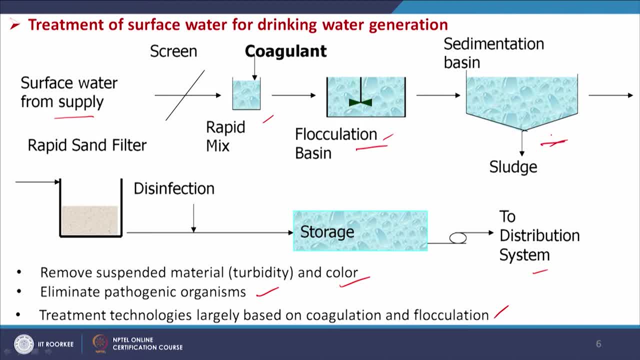 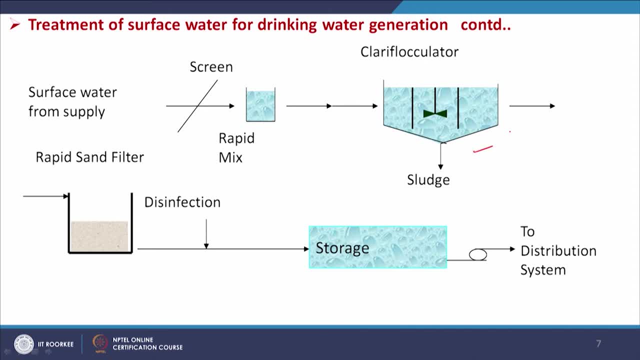 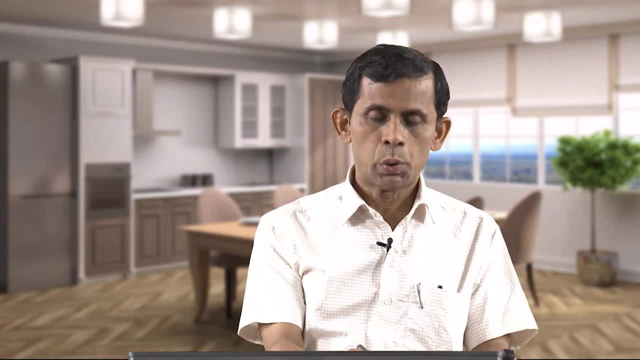 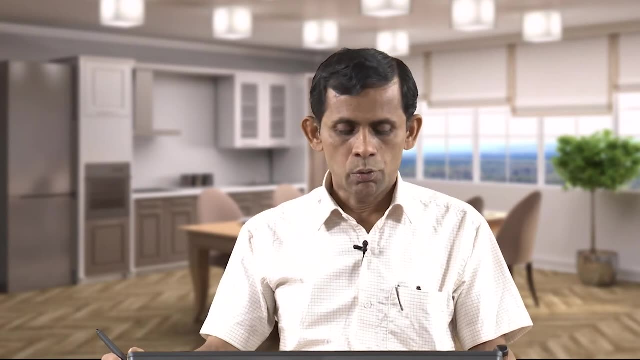 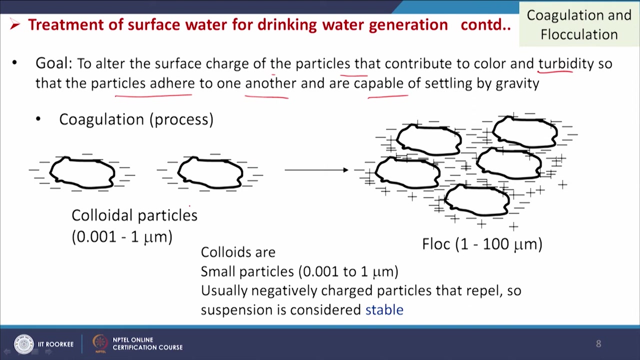 So very fine. particles will not be able to do show in the water solution or in the water. but if we add some coagulants or flocculants, then these charge neutralization can take place and the particles will be able to come closer. 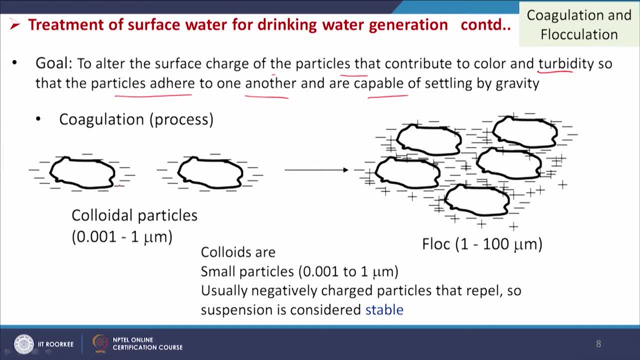 If we make some slight agitation, then it will become closer and a bigger agglomerate will form and that will be settled. and this is the mechanism for this. and colloids are small particles that is 0.001 to 1 micrometer. so this is the particles of 0.001 to 1 micrometer. 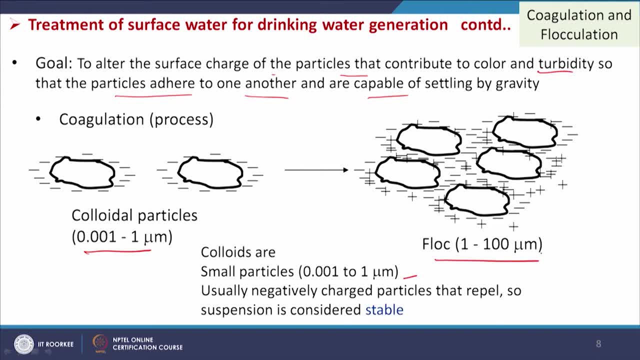 so after this coagulation process we are getting 1 to 100 micrometer, so say 100 times increment in the size, So now that small particles will be able to settle, so usually negatively charged particles that refill. So suspension is considered. 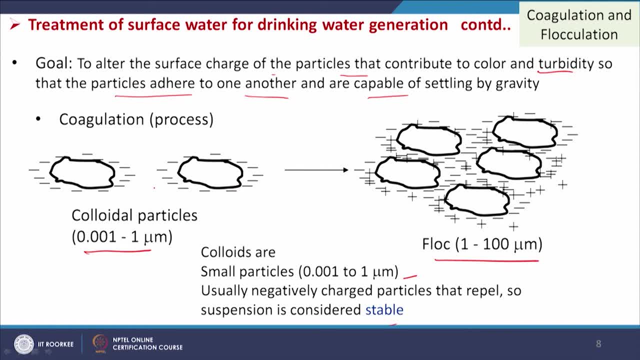 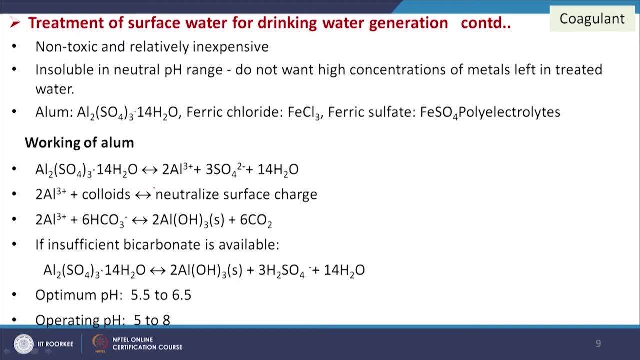 So normally these particles are stable, but when we add the coagulants so this stability breaks and it falls Now coagulant. how they work, we will see here and some common examples of these coagulants, like say, Al2SO4, whole 3,, 14H2O, that is, alum, and ferric chloride, FeCl3, ferric sulfate, FeSO4. 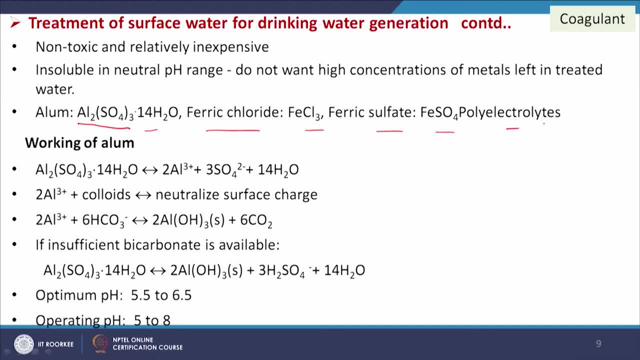 and polyelectrolyte. So these are the different materials which are used, and then these are normally non-toxics and relatively inexpensive. If it is toxic, we will never use it for the treatment because that will be dangerous for the health and insoluble in neutral pH range. do not want high concentrations of metals. 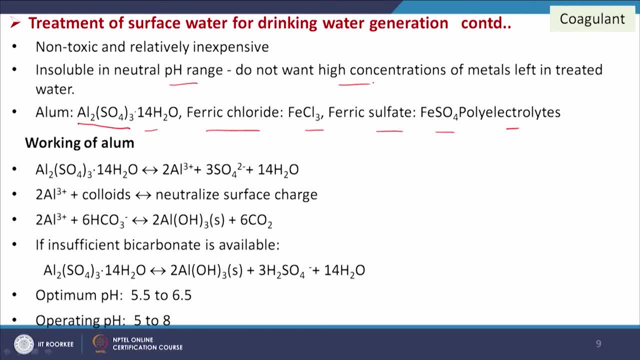 left in treated water and we will see the working here. So if we add aluminum sulfate, so Al2SO4, whole 3, 14H2O, so that will give us Al3 plus and 3SO4 2 minus plus 14H2O in the water. So that will give us Al2SO4 whole 3, 14H2O. So that will give us Al3 plus and 3SO4 2 minus plus 14H2O in the water. So that will give us Al3 plus and 3SO4 2 minus plus 14H2O in the water. 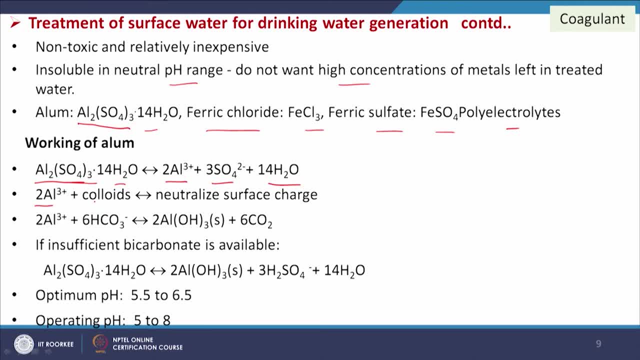 Cause of these two materials will help to neutralize the charges of the colloidal particles. so then, neutralize surface charges and then, if bicarbonate is present, so this will react with Al3 plus and AlOH, whole 3 solid will be formed. 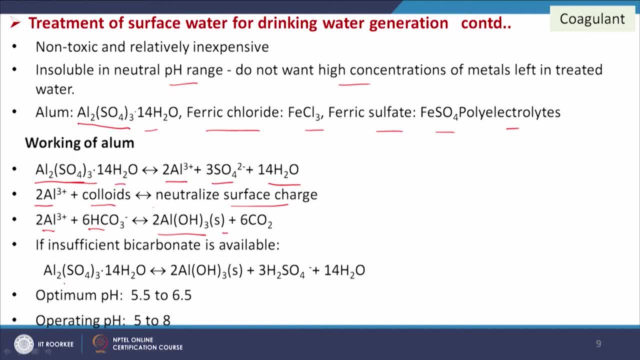 And if insufficient bicarbonate is available, then Al2SO4 whole 3, 14H2O will form AlOH whole 3, sulfur plus ThriH2SO4 plus 14H2O. Now, which are the binders? 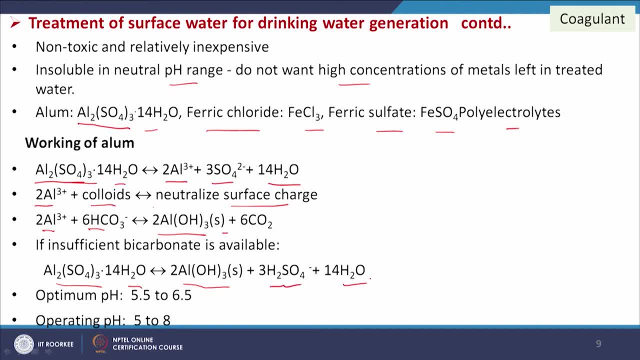 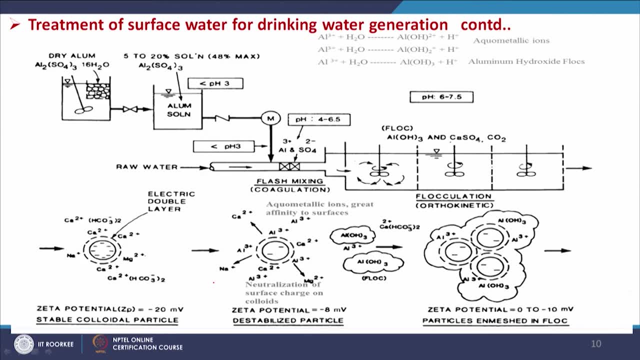 So the binding bonds are not copied. Now we will see how they are basically formed. This is a bishop, This is a block. Operating pH is 5 to 8 and optimum pH is 5.5 to 6.5, so this is for coagulation and we 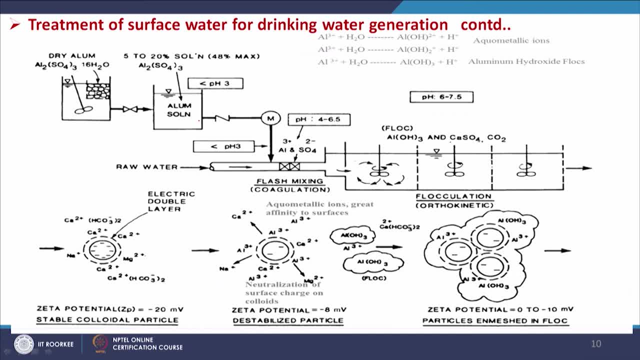 see here, when we are adding alum, here, alum solutions, we are coming to this raw water and here we are giving some slight agitation. so initially the flocculation takes place. So flocculation, then the particles becomes closer and this is a colloidal particles negatively. 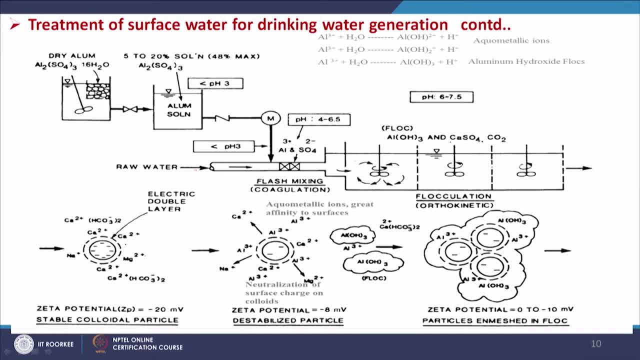 charged and some positive ions present in the water makes a double layer here. So this is a stable one. So now if we add some aluminum sulphide, so that will be converting Al OHol3 and then some Al 3 plus ion also, so that will disturb this. 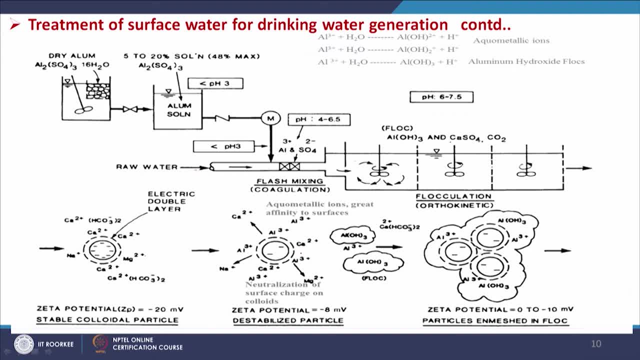 So the particles will be able to come closer and then, in this case, you see, the more number of particles are coming here and a floc is formed by this aluminum hydroxide. So this floc, and then it settles So very. 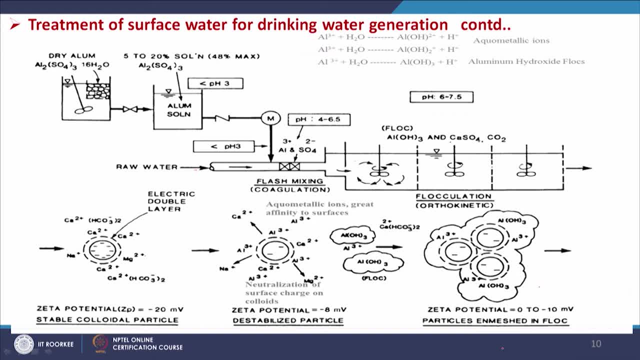 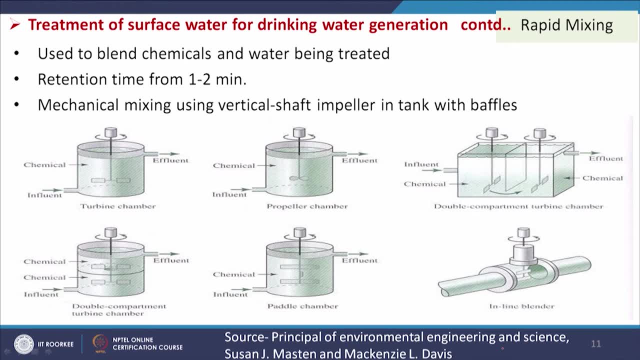 tiny particles are able to settle here. So both flocculation and coagulation take place in this unit, and then rapid mixing. So this is used to blend chemicals and water being treated, So rapid mixing is required. within small span of time the mixing will be done. 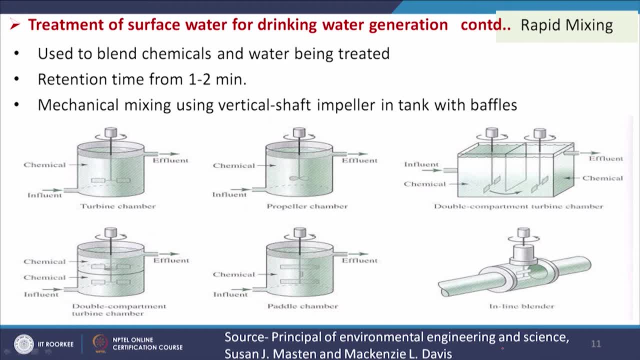 and then coagulation, flocculation will take place, then sedimentation will take place, And retention time for this is 1 to 2 minute. and mechanical mixing using vertical shaft impeller in tank with baffles. these are commonly used, So different types of rapid mixing. 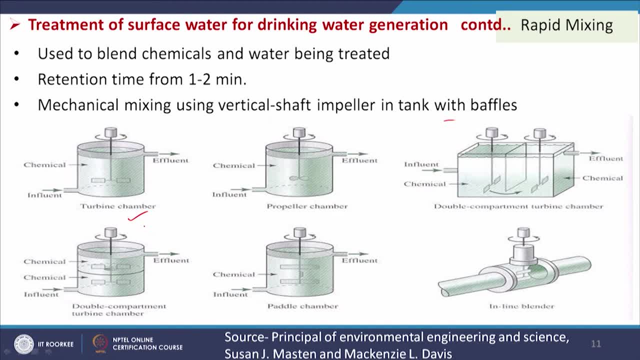 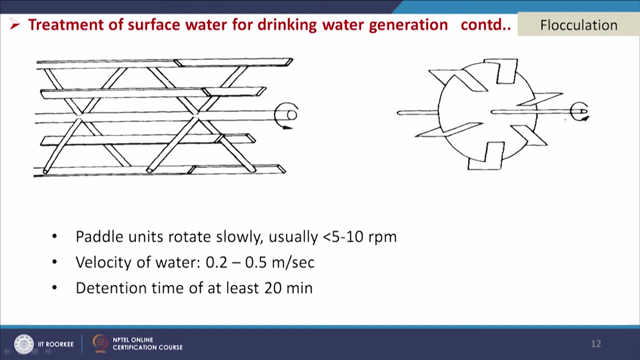 arrangement. you see, this is turbine chamber, propeller chamber, paddle chamber and it may be double compartment turbine chamber ON NUMBER OF TURBINED KETTLES And here double compartment turbine chamber, and inline collector is also there. So if we see, here the paddles are like this, So this is our central shaft, so this is our. 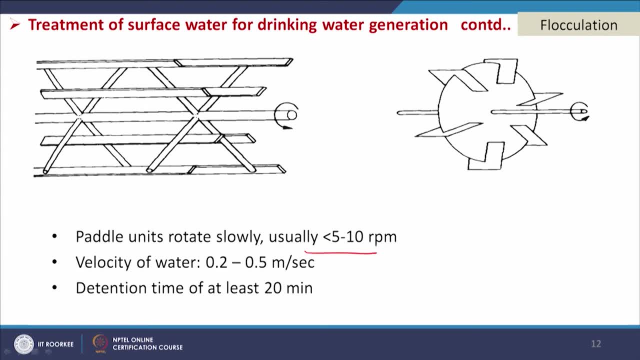 paddle. So paddle units rotate slowly, usually less than 5 to 10 rpm, and velocity of water is 0.2 to 0.5 m. dividers Then y Guild B steht bei cos cos Gluber avec Dahalienarnennah, warhardische Sterразmittschunze. 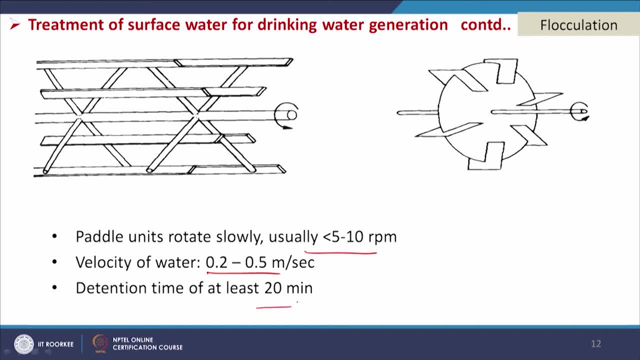 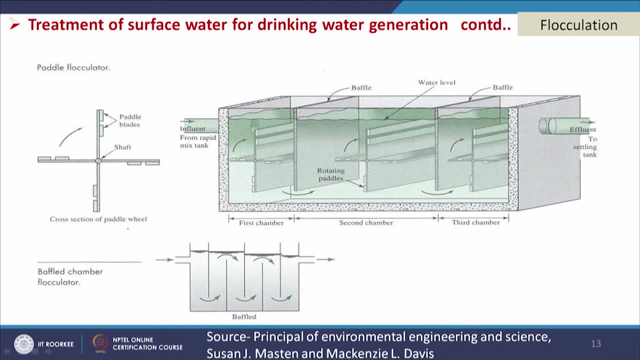 und der Grund sind sich für kallld realiziert. aber zum Croत來了, Here we point and back: meter per second and retention time of at least 20 minutes. So this is the conditions for flocculation. and then this is one say cross section of paddle wheel, and this is: 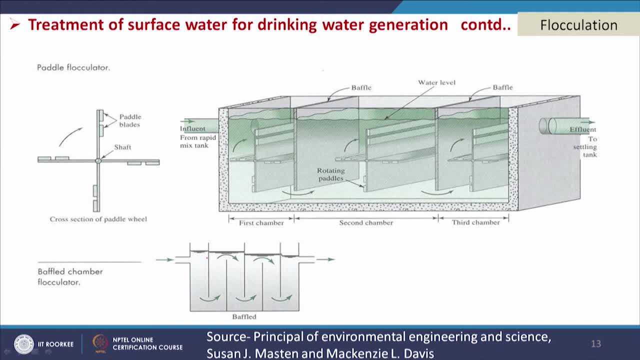 buffled chamber flocculator also is used, So the buffles are put inside the chamber and then say: here, water is coming. it will go like this, like this, So that way the efficiency improves. just, we have discussed in case of micro-settler, in case of sedimentation unit. 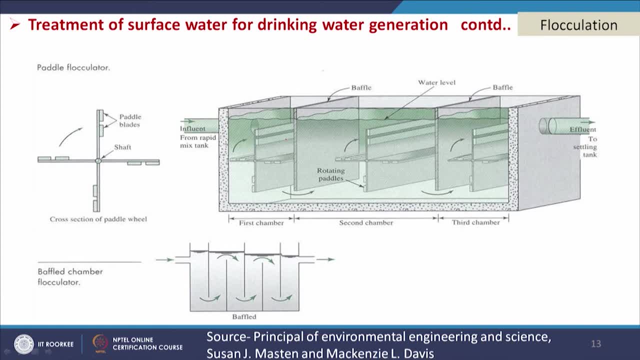 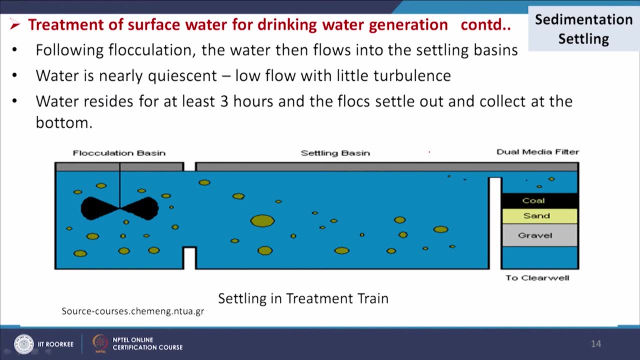 the similar way. this incorporation of this buffles also increases the removal of the particles. Then we are coming to sedimentation, settling or tank. So after flocculation the water then flows into the settling basins. So water is nearly quiescent, low flow, with little turbulence. water resides for at least 3 hours at least. 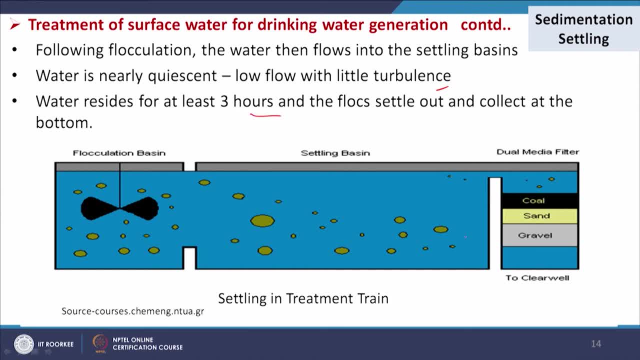 4 hours and the flocs settle out and collect at the bottom. So this part is our, this is flocculation. So then it is coming to settling basins. So flocculation, settling basin, then it is coming to further filtration. either you can. 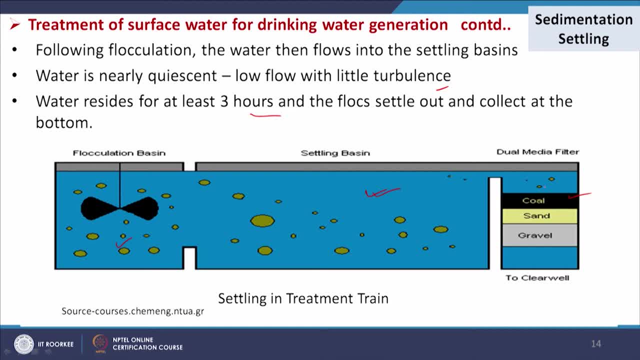 use sand. we can use multimedia or dual media filters. So here, just like say, coal, sand, gravel is shown. that is your multimedia filters. So this part is with related to settling. So we provide. 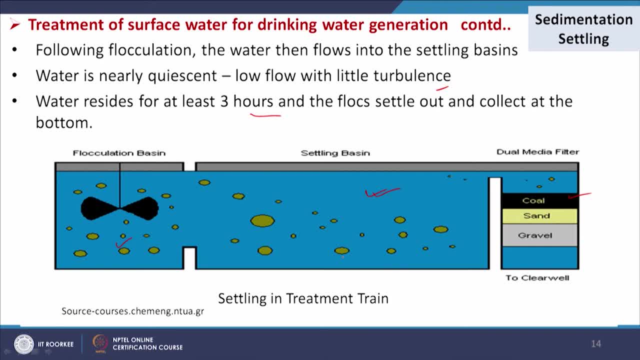 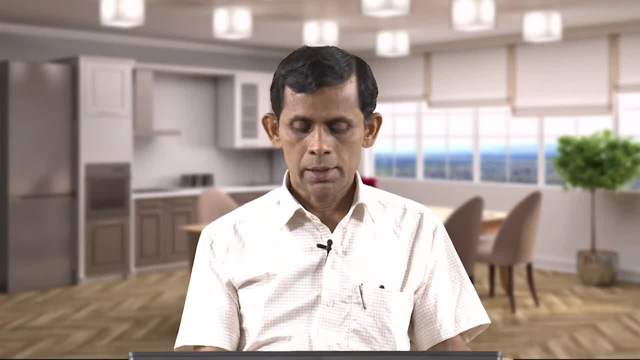 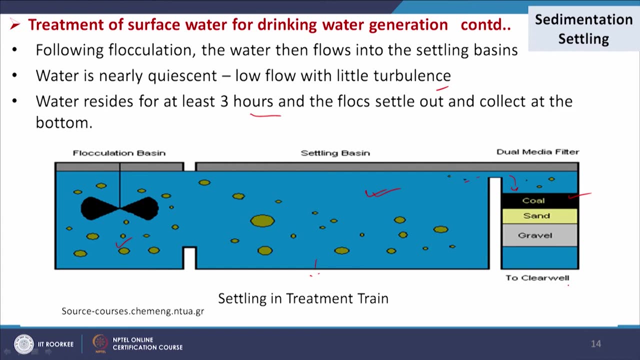 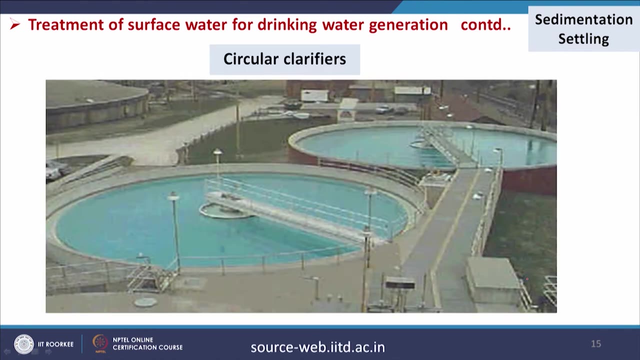 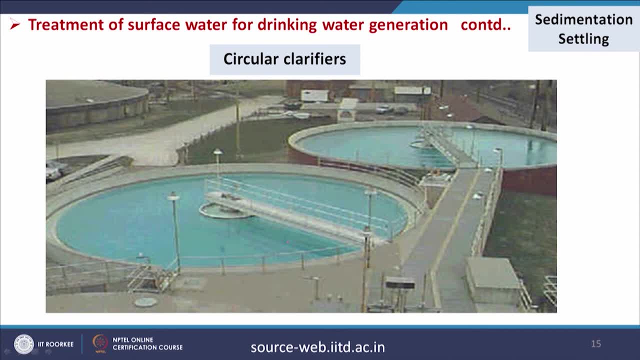 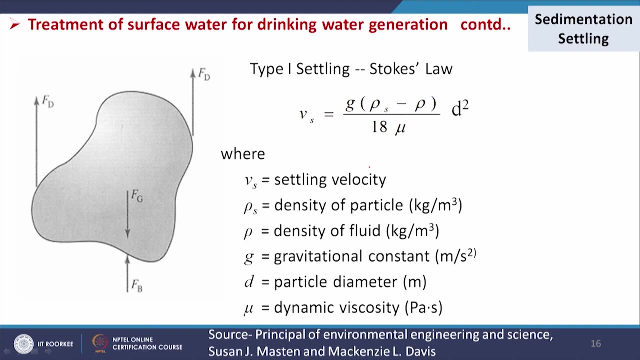 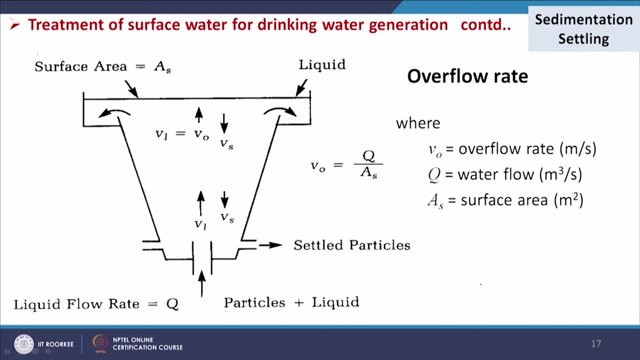 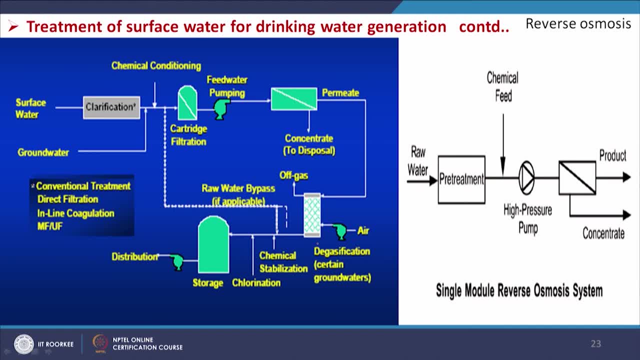 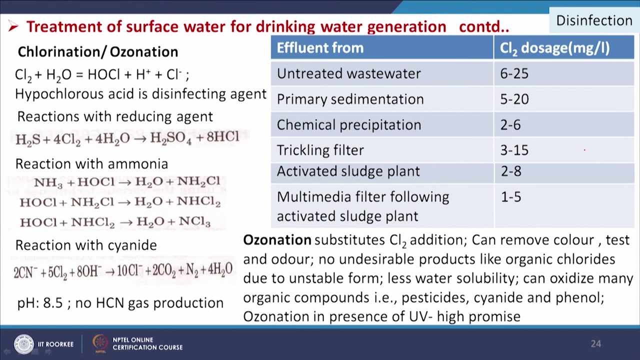 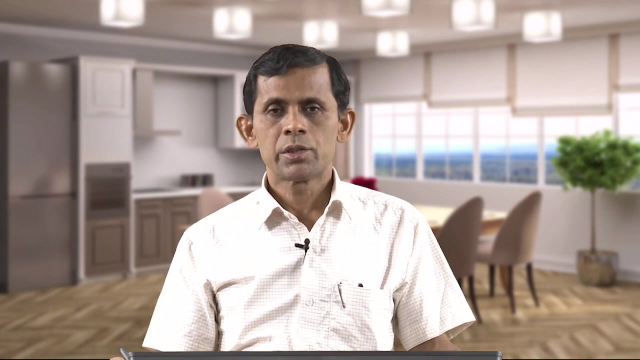 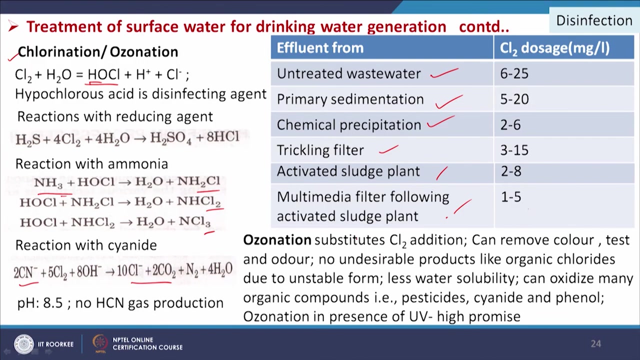 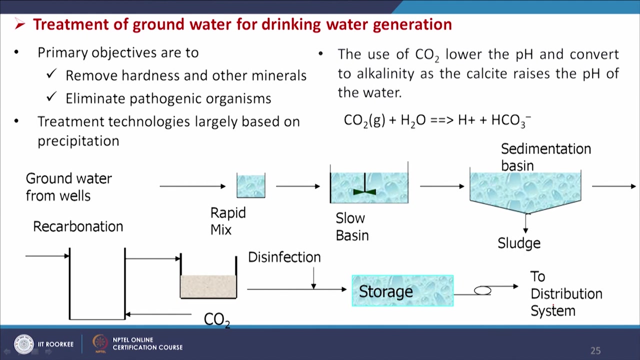 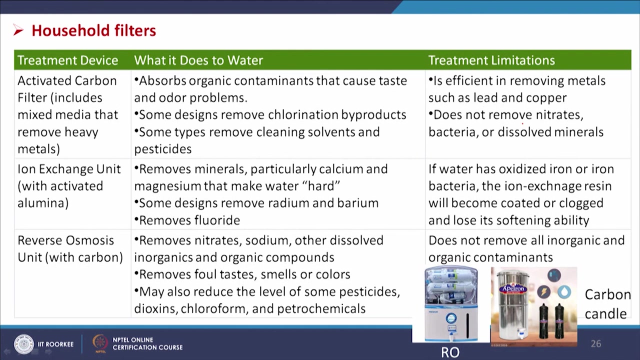 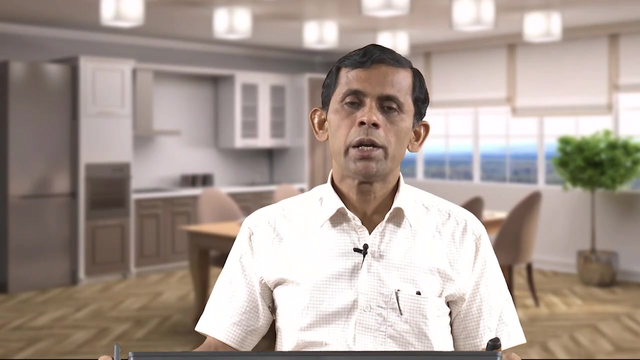 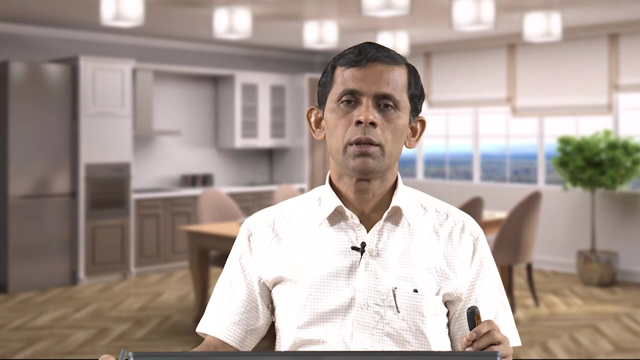 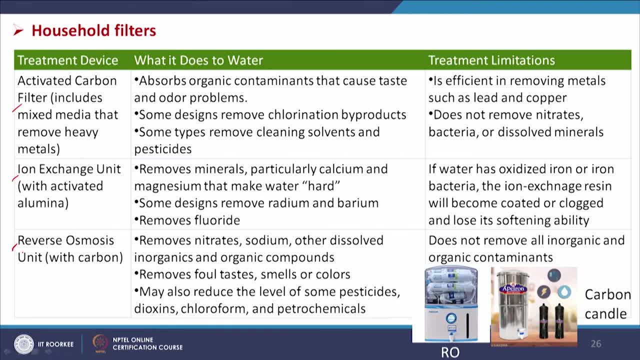 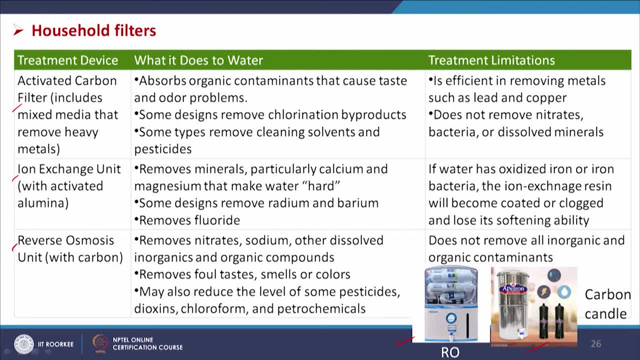 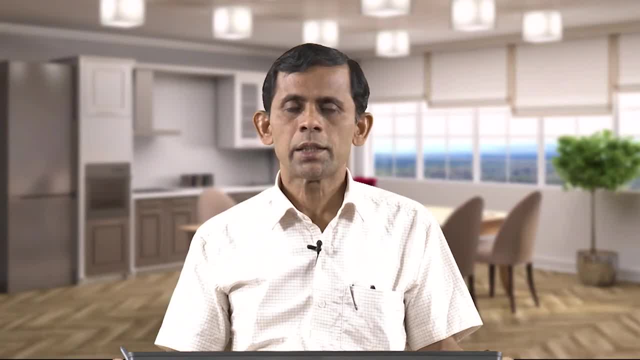 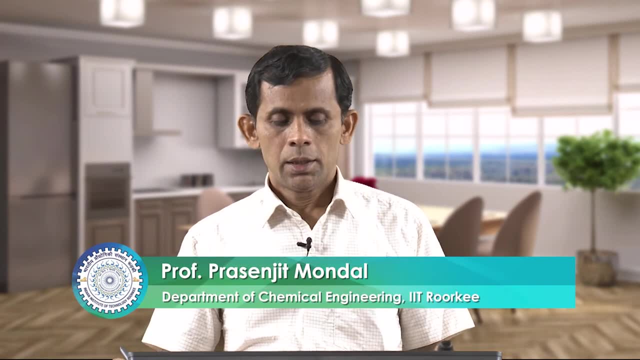 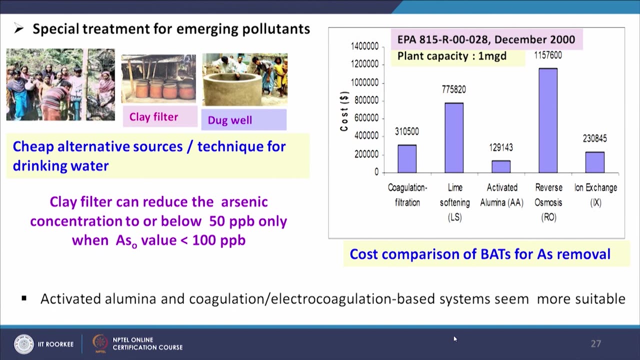 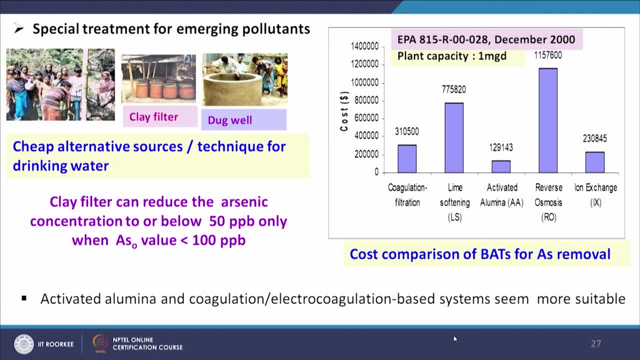 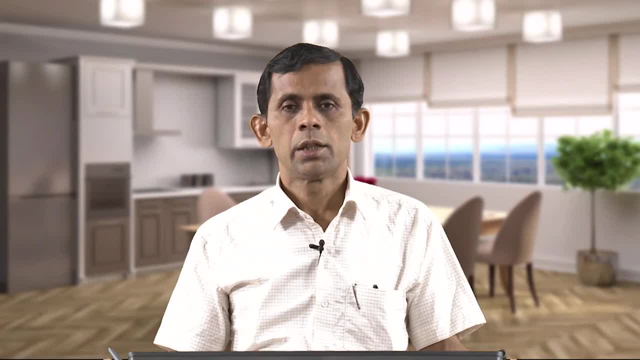 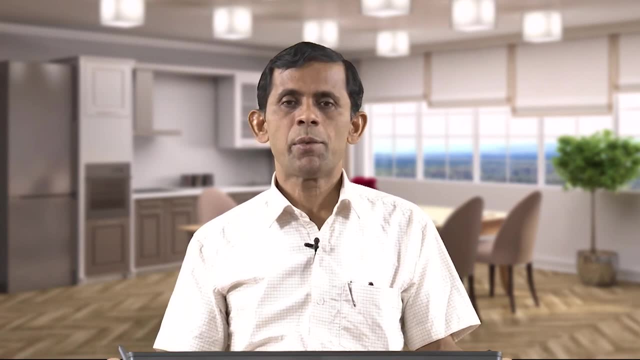 which is being contaminated by different human activities or from the natural sources like, say, arsenic, fluoride, pesticides, uranium, etcetera. So all those chemicals are emerging in nature and we need to have some special treatment. apart from the discussions which we have made, those treatments may not be applicable or 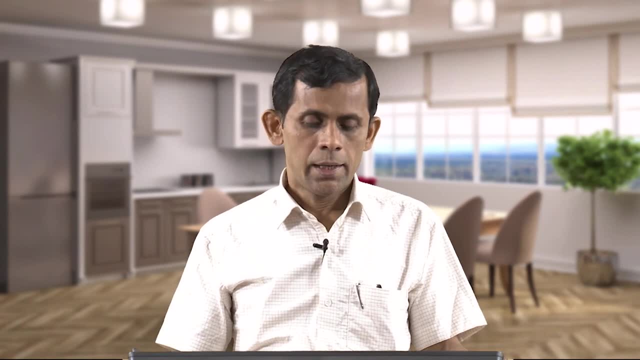 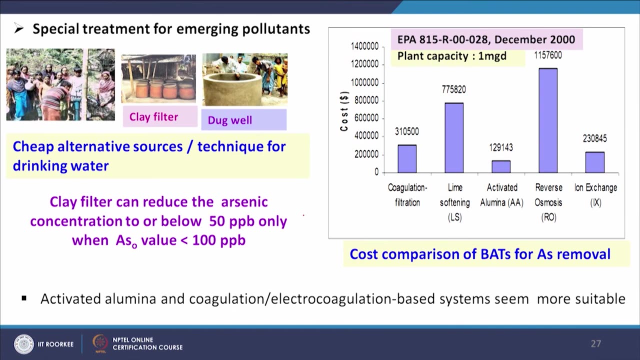 suitable for the treatment of this type of pollutants. And if we see the literature then we see that for a particular arsenic and fluoride removal, for arsenic removal. so in India people opt for different low cost technology. but these technologies are not that efficient and best available technologies are available at far 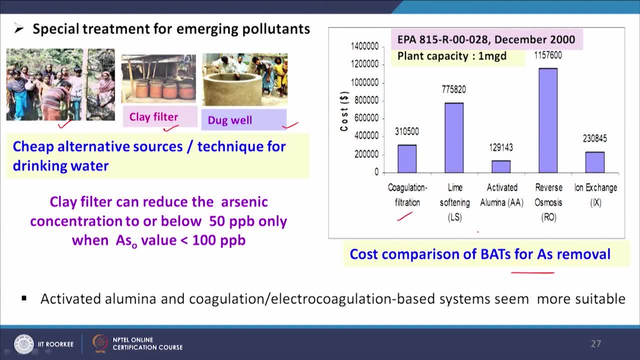 EPA, That is, coagulation and then lime softening, activated alumina, reverse osmosis and ion exchange. these five are identified as the most promising And out of these the…. We see activated alumina and coagulation or electro coagulation. these two techniques are